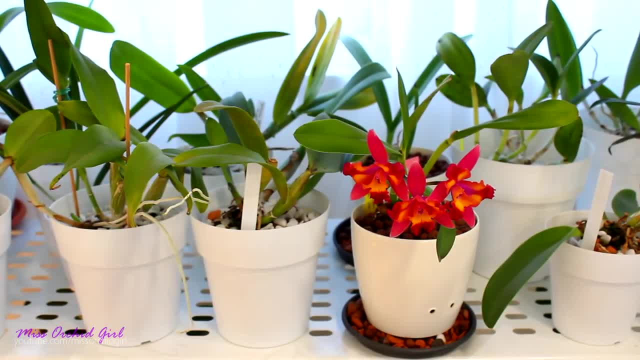 go through the most popular orchids you can find at the flower shop. for those of you who don't have experience in identifying at least the family of orchids just by looking at the other structures of the orchid, So we'll do that really fast and then we're gonna take a case. 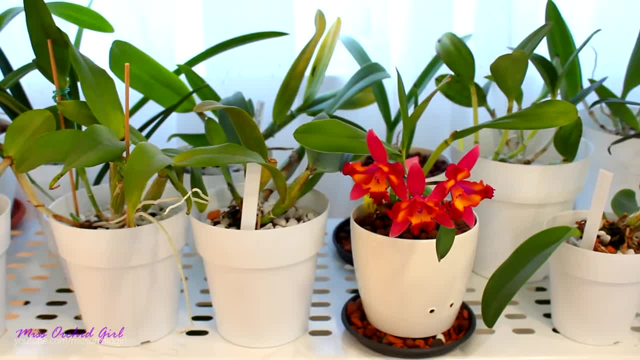 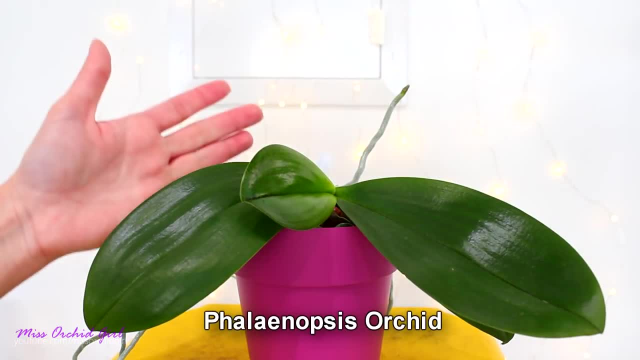 an orchid that I recently purchased at a discount and go through the motions and tell you how I care about it until it blooms. and I figure out what it is. First of all, the Phalaenopsis orchid. It is the most popular orchid in flower shops at the moment, So it is to be expected that you will. 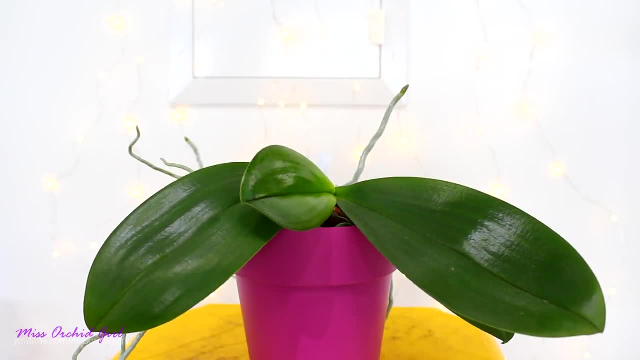 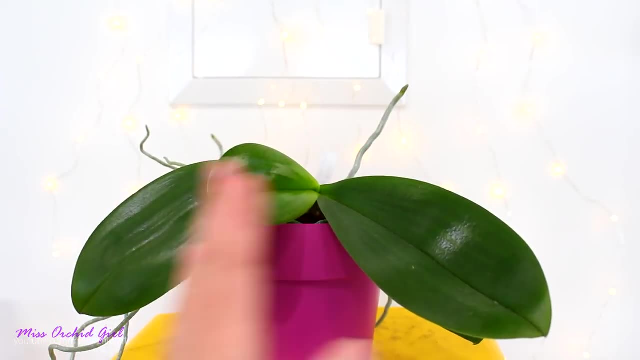 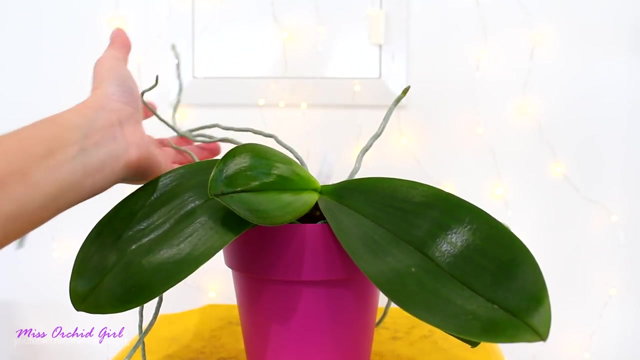 find this orchid on the discount rack as well. It's easily recognizable. it doesn't have any pseudobulbs. it has a central axis. Also, the leaves grow sideways, mirroring each other, and of course, the Phalaenopsis have thick fleshy roots that sometimes can grow in the air Overall. 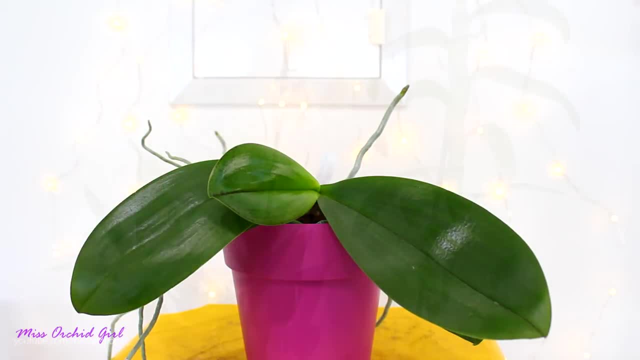 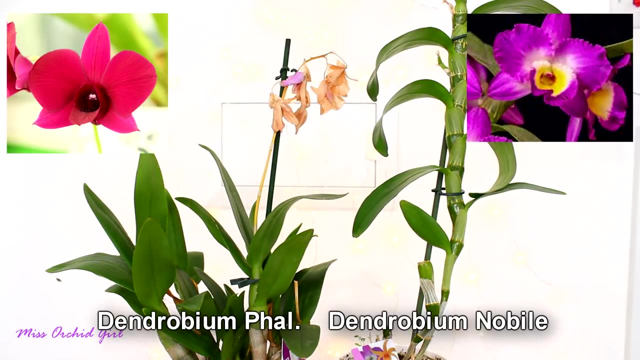 you don't really have a problem in identifying the Phalaenopsis orchid family. Then we have the Dendrobium orchids- Yet again very popular orchids in flower shops and garden centers, And we do have two types of Dendrobiums. Sometimes you will be lucky and the name will be on the tag. 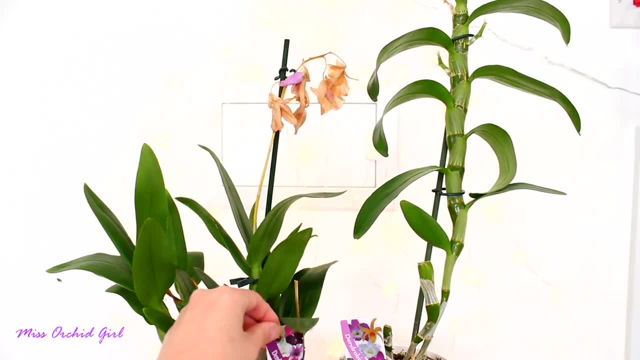 but this is pretty much 5% of the cases. Most of the times you will have either a tag saying just Dendrobium or orchid, and that's about all you'll get. It's easy to spot a Dendrobium because they. 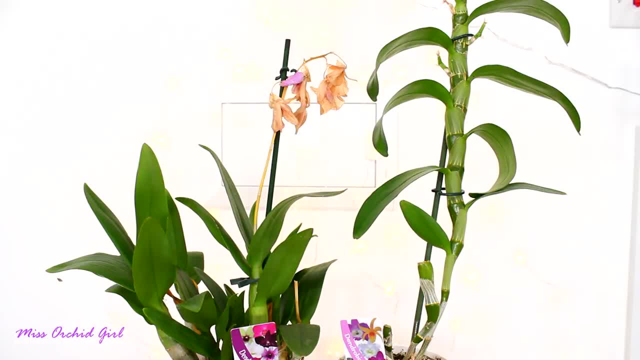 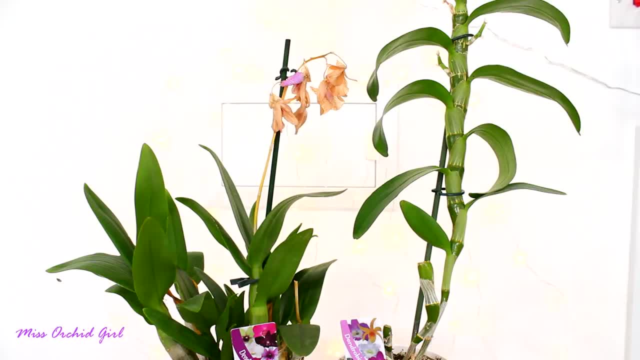 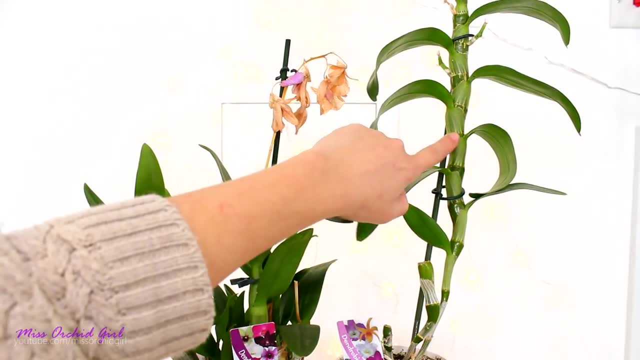 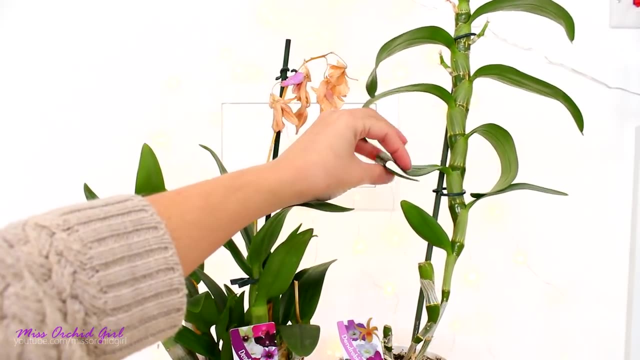 canes And, as I was saying, there are two types of Dendrobiums. One is the Nobile and you can recognize it by its cane and the foliage On the cane. you will have sections that are glossy and sections that are matte. Also, the leaves are very thin and very, very flexible. You can totally do. 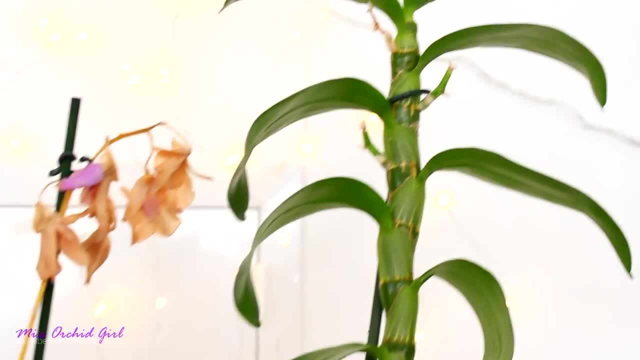 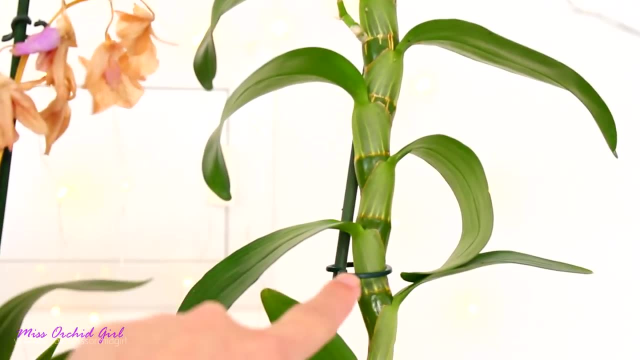 this without harming the leaf in any way. Also, if you look at the top, you will see where the flowers used to be, Depending on the Dendrobium. you will find these little stumps all across the pseudobulb, or at least only at the top, And this is because the Nobile Dendrobium flowers 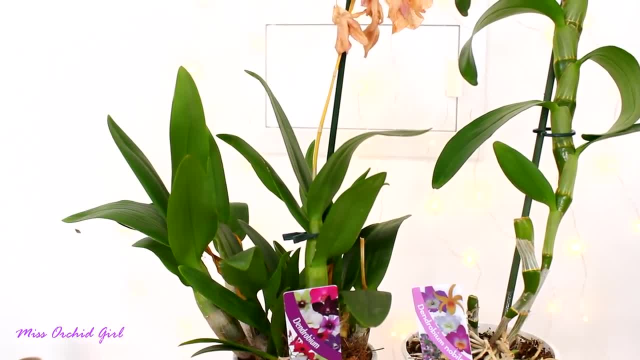 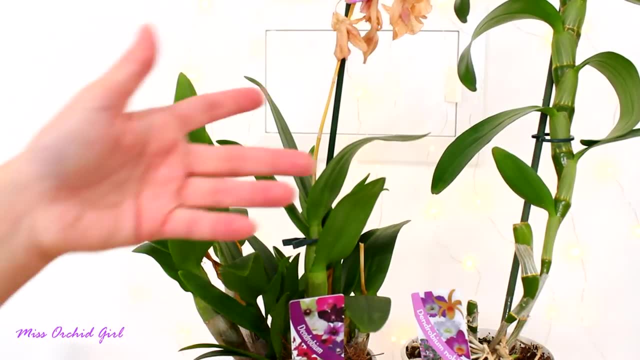 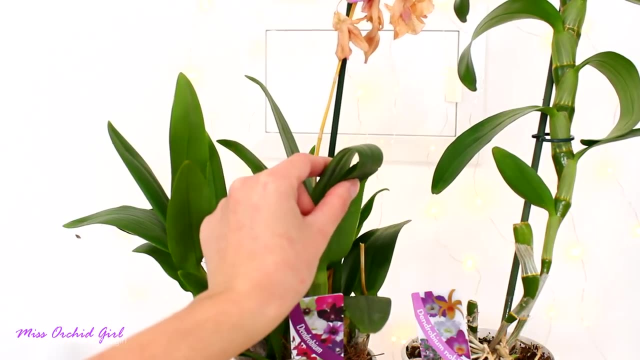 along its cane. The Dendrobium Phalaenopsis is quite different. You will not see glossy pseudobulbs. They are pretty much matte for the entire length. Also, their leaves are a lot stiffer, Even if they might be quite flexible as well, you cannot bend them all the way. 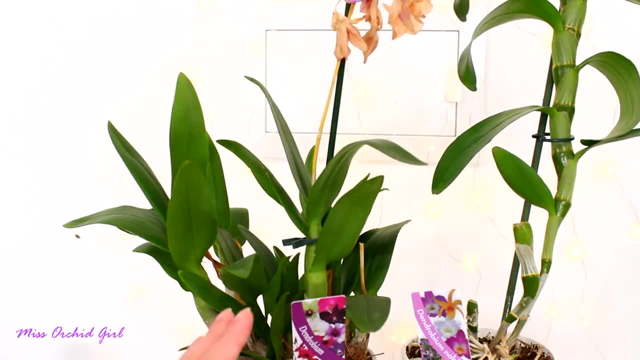 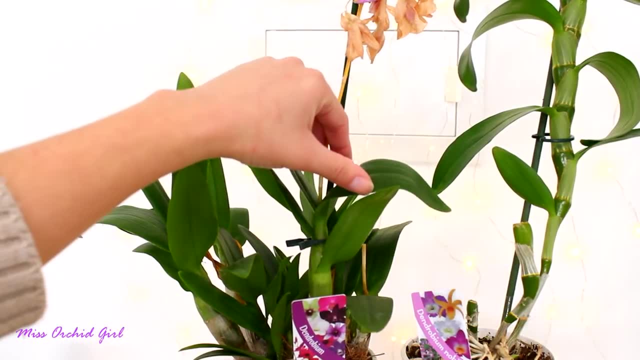 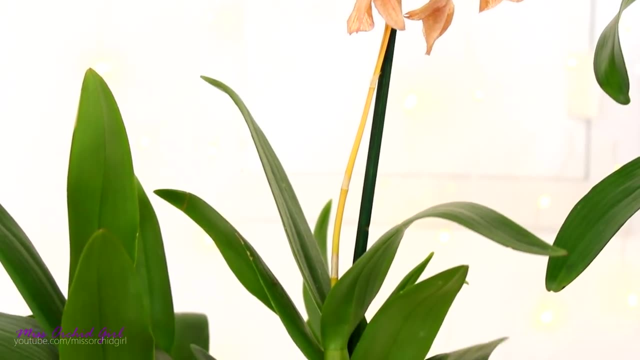 And if you try you will definitely snap them. Some Dendrobium Phalaenopsis are shorter but others are longer, So size of the cane doesn't really matter, But on top of each cane you will see the remains of the flower spike. Dendrobium Phalaenopsis produce long flower. 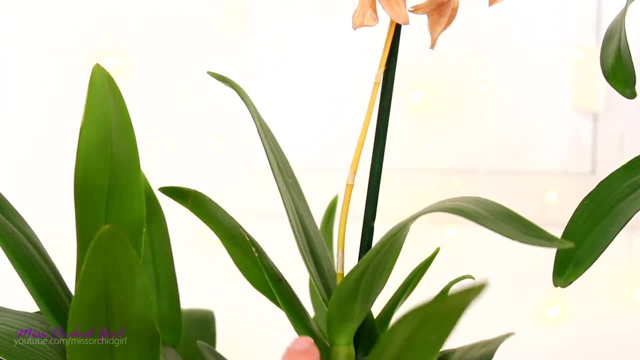 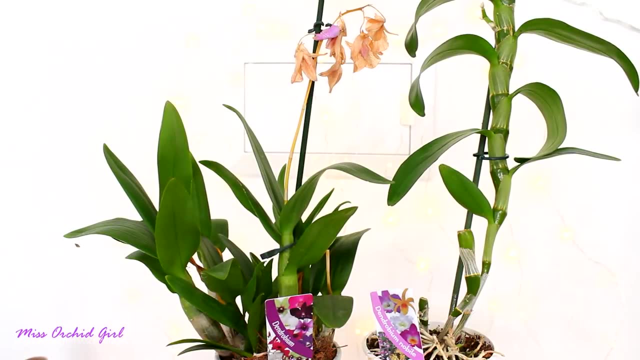 spikes that arise from the top or one of the nodes in between the leaves. Mainly, though, they do bloom from the top of the cane. Either way, I think it's pretty easy to recognize a Dendrobium, and even go the extra step of identifying if it's a Nobile or a Phalaenopsis type. 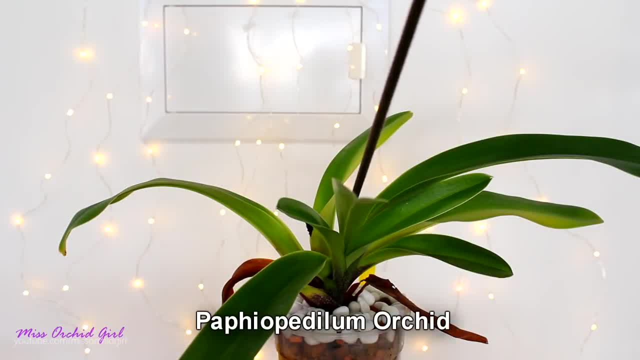 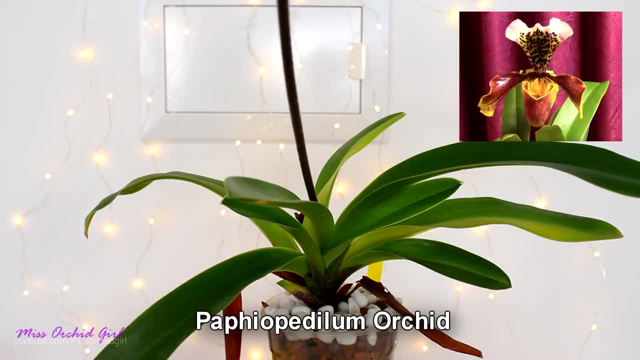 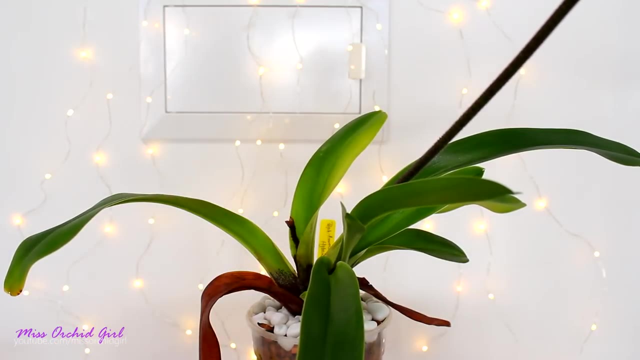 Another common orchid you might find discounted in flower shops is the Paphiopedilum, And at first glance it looks like a Phalaenopsis, But there are some major differences. Phalaenopsis orchids- the vast majority of them at least- do not bloom from the crown, from the center of the fan. They 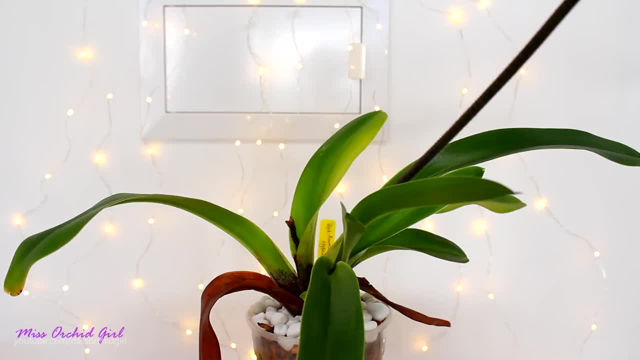 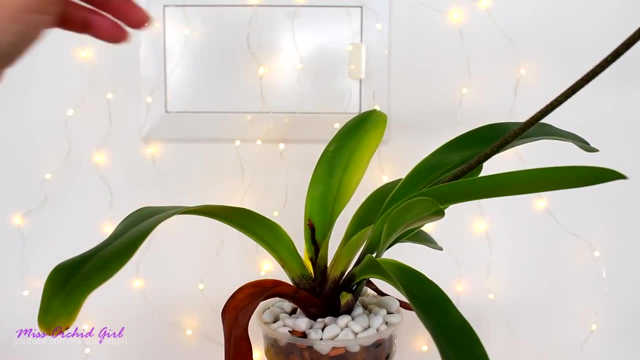 rarely produce a terminal spike, And that's a whole different story. It's not necessarily normal kids. So, as you can see, we don't have canes or pseudobobes, but we do have fans. And this orchid is actually not a monopodial, It is a sympodial. It just doesn't produce pseudobobes. Look for the 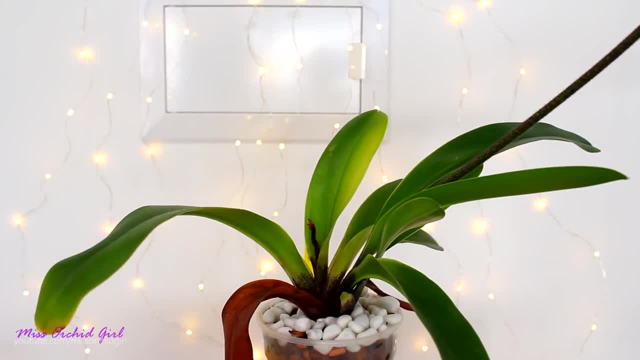 shape of the leaves. They're usually thin and elongated. When you look at a Phalaenopsis, you will notice the leaves are broader. Also, look at where the old flower spike was. If it's in the center, most probably it's a Paphiopedilum. Sadly, Paphiopedilums do not come in transparent. 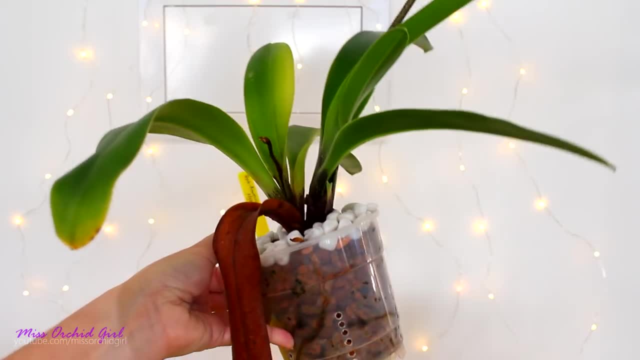 pots because they are semi-terrestrial orchids. But if you look at the leaves, you'll notice that they are very thin and elongated. But if you look at the leaves, you'll notice that they are very thin and elongated, But when you repot it and you see that the root system is fuzzy and brown. 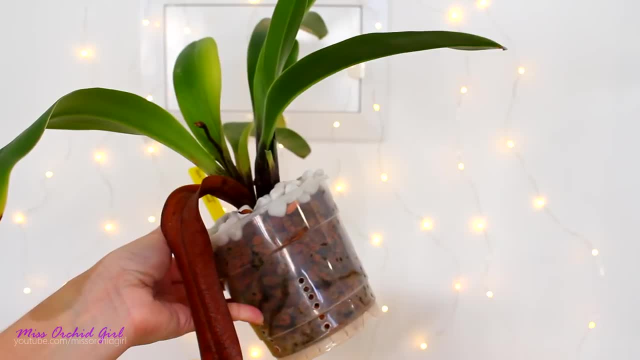 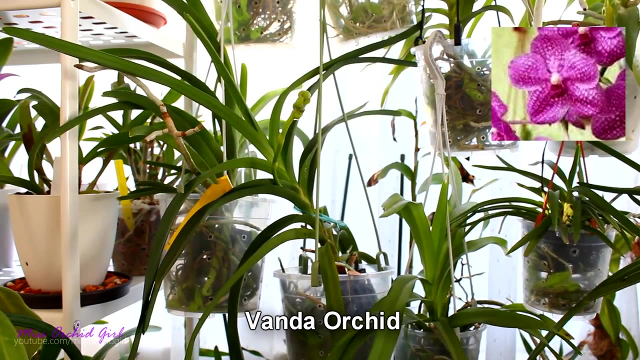 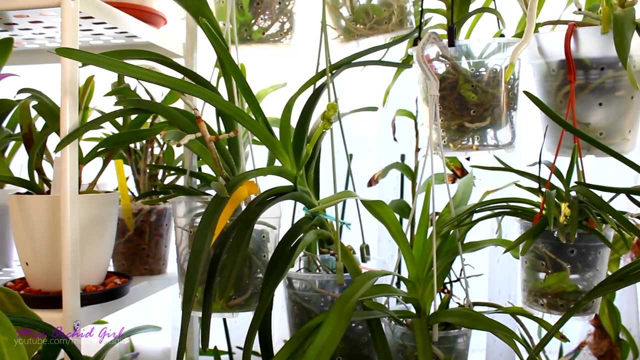 then you know you have a Paphiopedilum and not a Phalaenopsis orchid. Now, Vandas are the easiest to recognize in the sense that they're the only orchid available on the market without being potted. Vanda orchids are available either in little baskets either in those glass vases. It's. 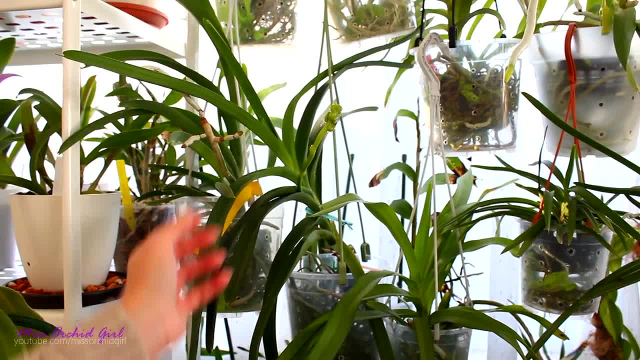 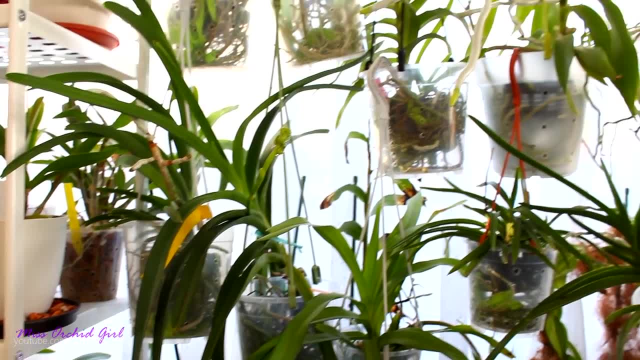 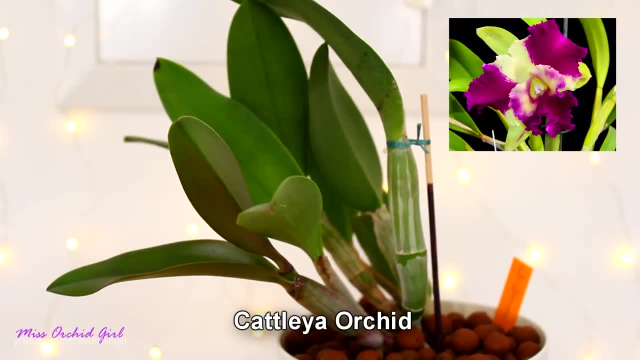 really easy to identify them. They're usually big. They don't have pseudobobes, They have long side leaves and a tall stem, not to mention exposed roots. So when you see a Vanda you just know it's a Vanda. The next orchid you can find in flower shops is the Callia orchid. It is slightly similar. 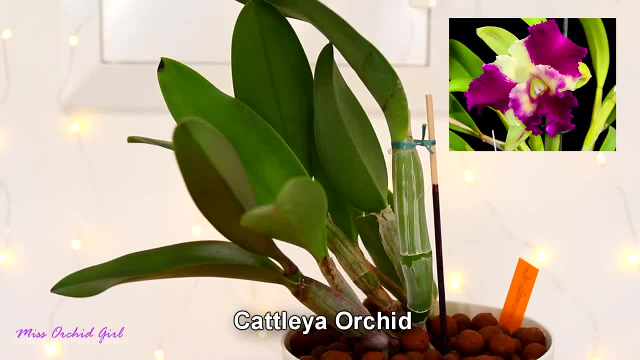 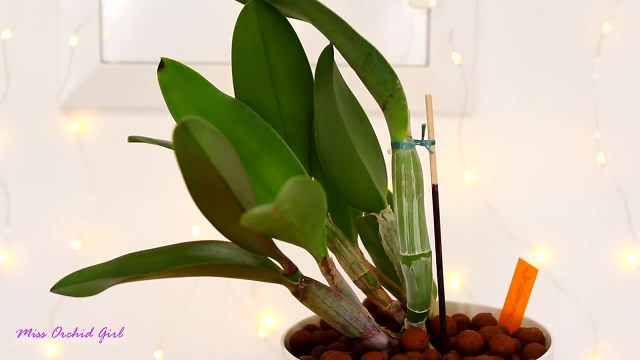 to the Dendrobium in the sense that it produces pseudobobes which are elongated and they look like canes, But on top, as you can see, we can have one or two leaves. for the main part. There are a few varieties that have more, but they're not many, Unlike the Dendrobium. a Callia orchid. 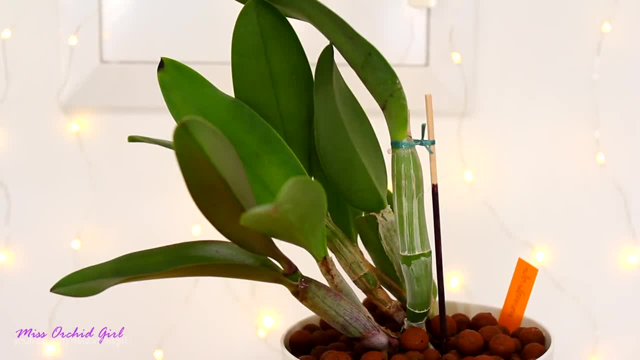 doesn't have multiple leaves towards the top of the pseudobobe And also in some cases the pseudobobes can be super, super plump and wide. There is a bit of variety. In other cases the pseudobobes can be quite thin, Callias can be small or big, But the ones you can easily find in 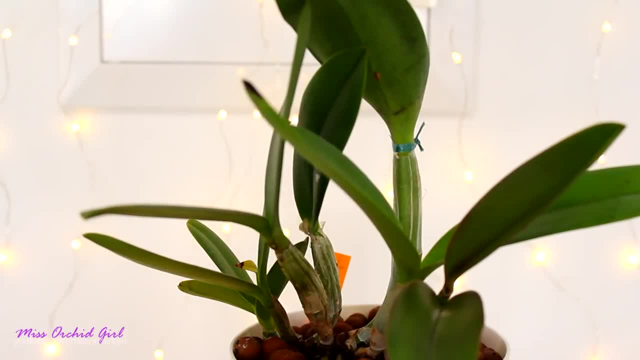 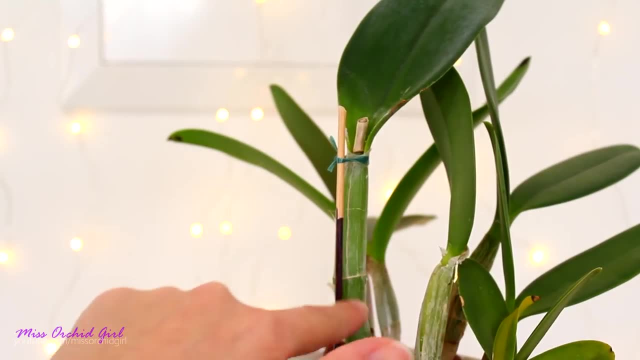 flower shops or garden centers always bloom from the top, So look for remains of flower spikes or sheaths from the top. Callia orchids never bloom from anywhere on the cane. There's a special species that does that, but most probably you will not find it in flower shops. 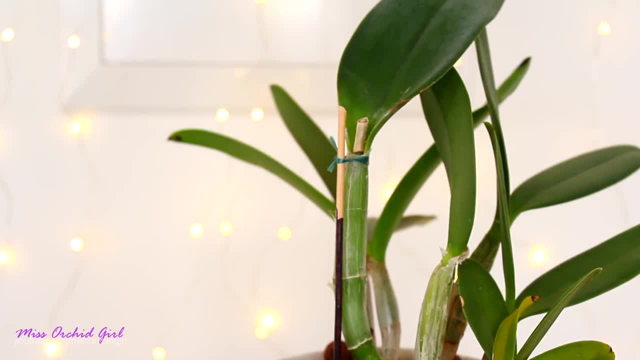 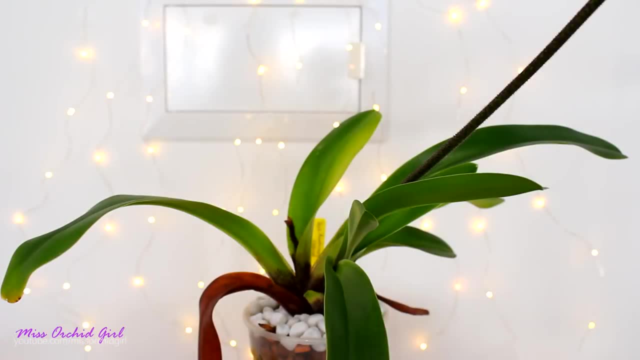 Even though Callia orchids can appear to be slightly similar to Dendrobiums, they really don't look alike, And now that you saw them in a video, I hope you can make the distinction better. All of these orchids that I just showed you, I think they're easy to identify, And down below, 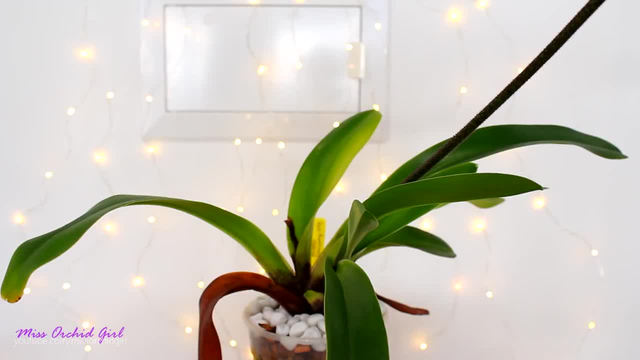 in the description. you do have care tutorials for all of these orchids, minus the Dendrobium Phalaenopsis. It is in the works, But check the description down below if you want to learn more about the Dendrobium Phalaenopsis. and if you want to learn more about the Dendrobium Phalaenopsis. 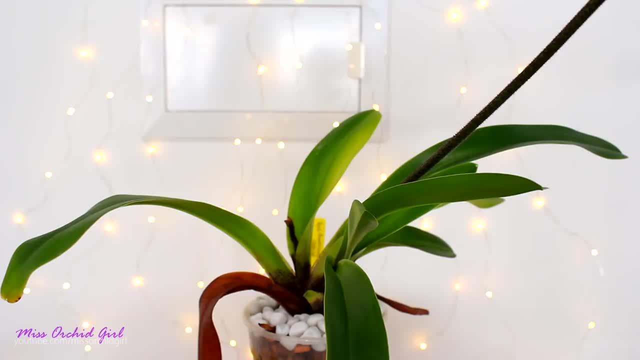 you can check the description down below. So even if you don't know exactly the color of the Phalaenopsis, they're all pretty much alike: Dendrobium nobilis. yet again, it doesn't matter what type of color it has- Most of them, if not all of them, they're the same and they require. 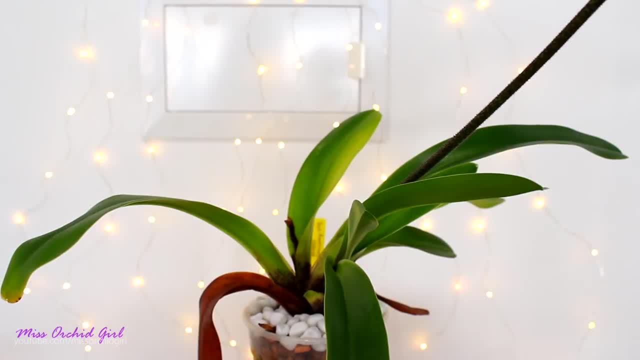 the same care. Dendrobium Phalaenopsis: same story. Paphiopedilums, the ones you find in flower shops- same story. You can care for them pretty much in the same way, Because most of these orchids. 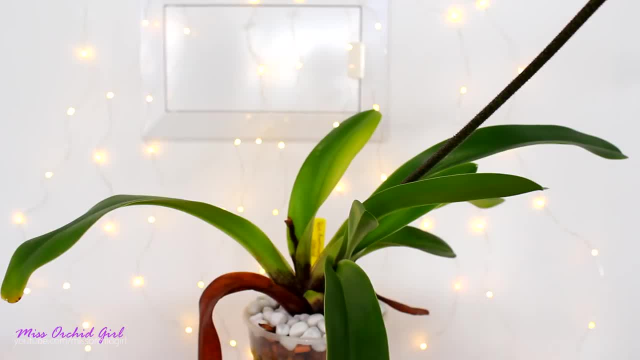 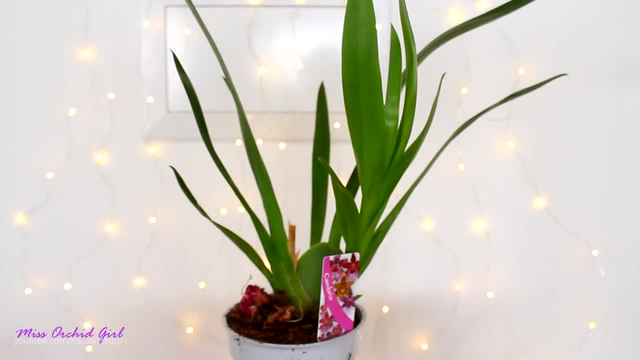 they're in centers and without a tag, because they're mass produced, They're easy to grow, they're meant for home growing. All with the exception of one particular family, the Oncidium or Oncidium intergeneric. There are hundreds upon hundreds of varieties of this orchid, and the bad 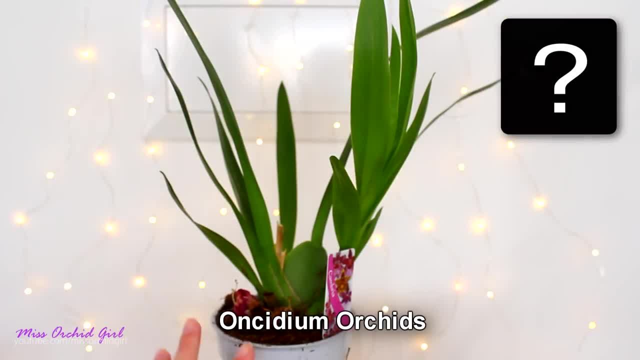 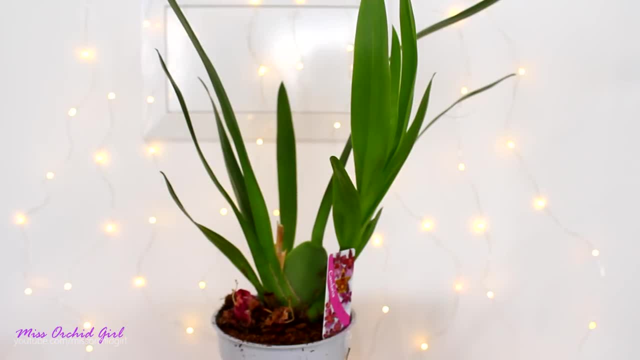 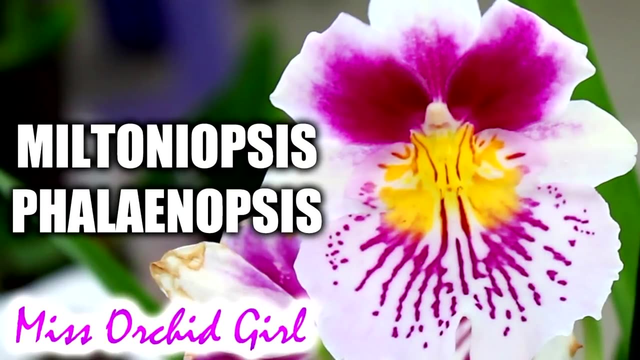 thing is they don't all take the very same care. Now, overall, these orchids are not necessarily not meant for being grown in a home, but there are a few that are certainly, in my opinion, not meant for the conditions, And these are the Melitoneopsis and their hybrids. They're a special case of 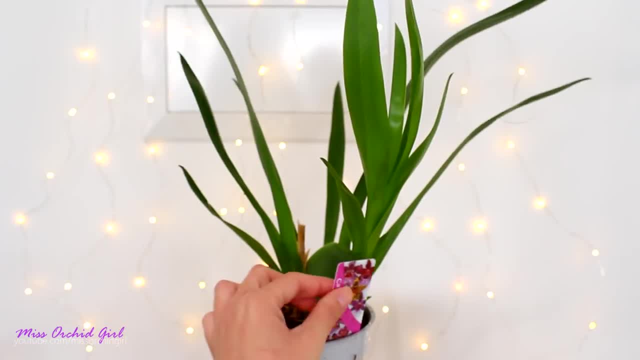 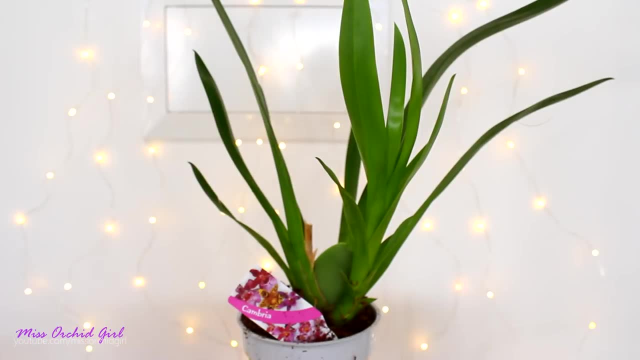 Oncidium-type orchid. Oncidium-type orchids and their hybrids pretty much all look like this: They have a roundish or elongated pseudobulb, they have green stripy leaves and there are very subtle differences in between them. So, especially when you're at the beginning, you cannot say if this. 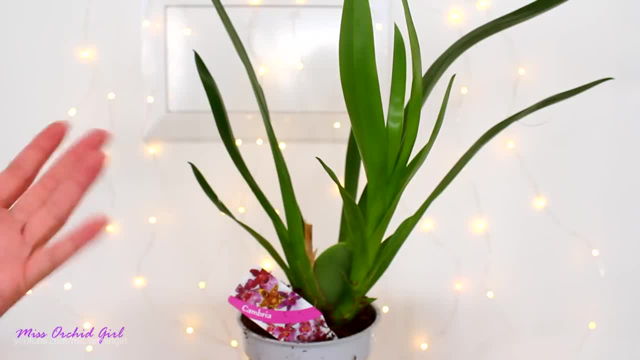 orchid is an intergeneric, an Oncidium, a Boracea, a Melitoneopsis, whatever. Here in Europe sometimes we call them Cambria. It's just a commercial name that specifies to us this is not an Oncidium. so this is good, But I've 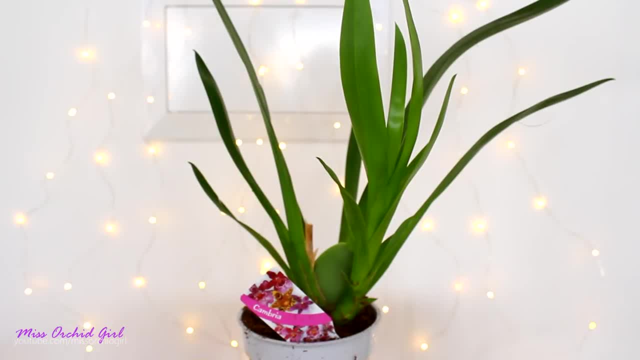 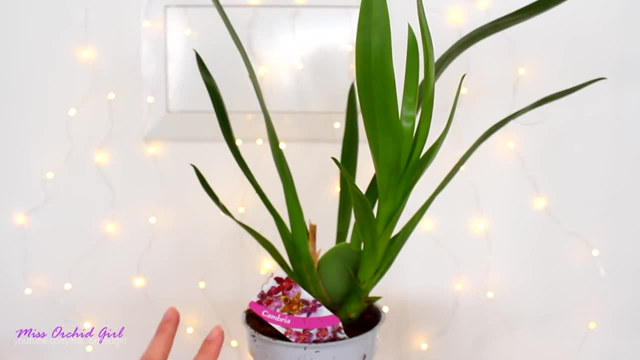 seen Oncidiums with the tag Cambria as well, so it can be slightly confusing. I'm not entirely sure how it is in the USA and what the tag says, but the Oncidium and Oncidium intergenerics family is. 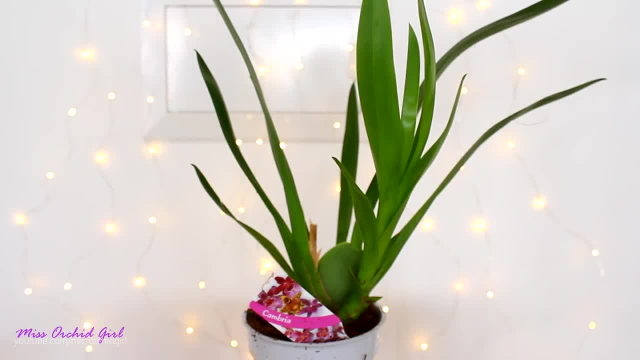 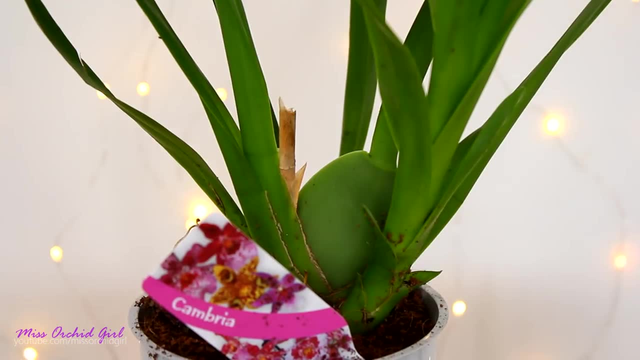 just so diverse it can be pretty, pretty counterintuitive. So, as you can see, the orchid we have in front of us today apparently is an intergeneric. What intergeneric, I am hoping to know, because I have experience, but let's presume that we don't know. 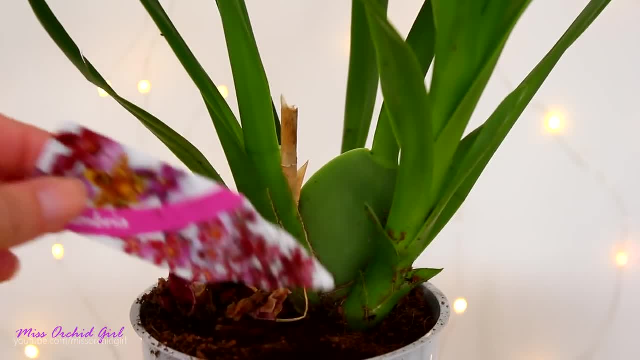 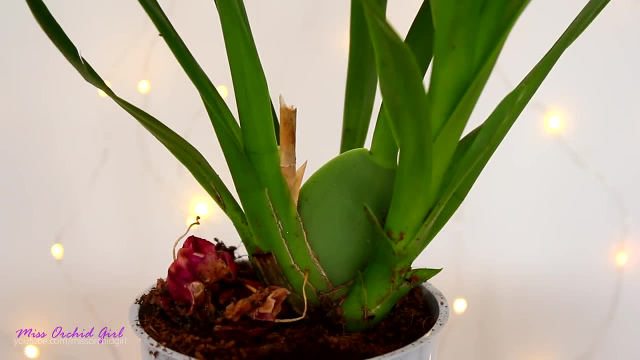 What is the first thing we need to do? Well, first of all, we need to put this orchid somewhere in our home. How do we choose a place? Choose the safest place possible. At this point, preferences of the orchid don't matter all that much. We're gonna try to find the range that can accommodate. 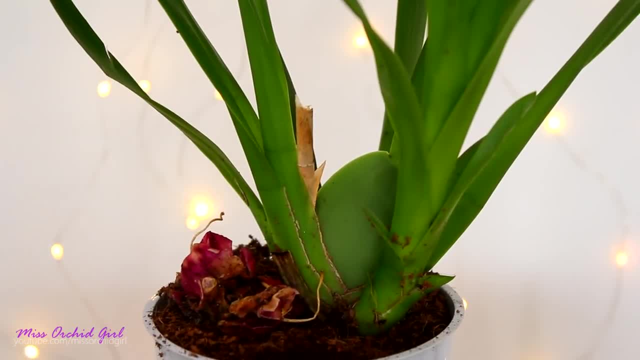 most of these intergenerics. So find a place in your home that is not very warm or very hot and it's not very cold either. It's somewhere between. If you're pretty comfortable in the house, it should be comfortable as well. At the same time,